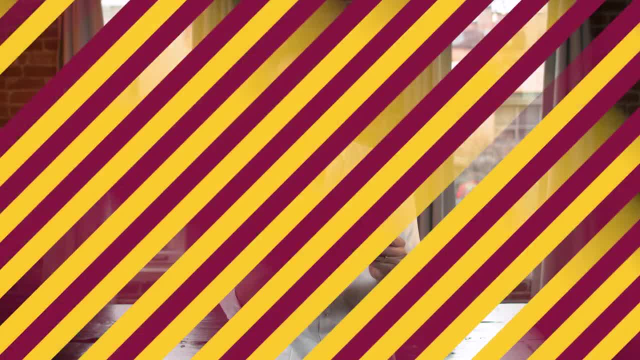 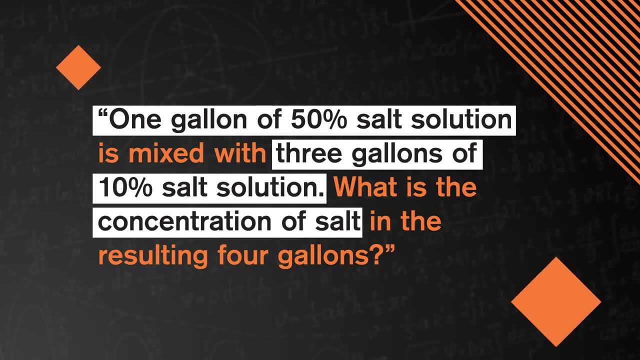 if I quickly can sort my little book of word problems. Let's see: One gallon of 50% salt solution is mixed with three gallons of 10% salt solution. What is the concentration of salt in the resulting four gallons? Hmm, As you might be able to see, I'm a little flustered, But I'm going to acknowledge my. 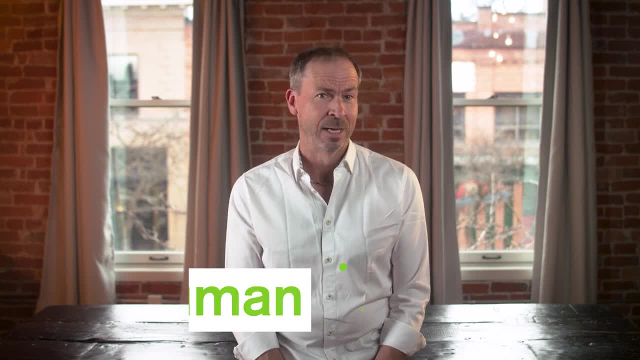 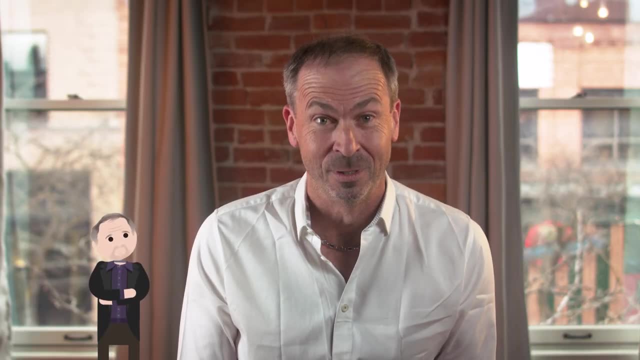 emotional reaction, because how I'm feeling influences my problem solving, And that's the first step: Be human. I'm feeling a little alarmed and unprepared. Now I was talking quite confidently about word problems in general, But now that I have a specific example, I'm at just a bundle. 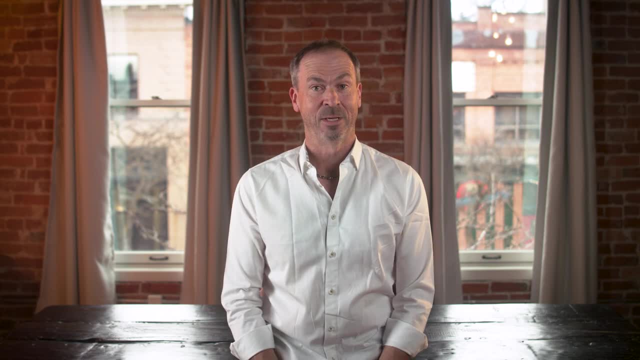 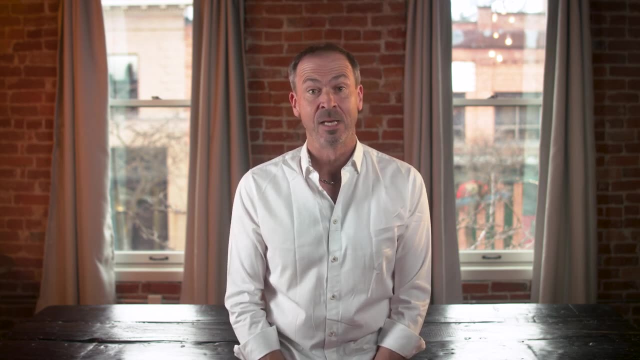 of nerves, And that's okay. Mathematics is a human experience, not just computations. If you're nervous about a problem, you might skip over important information when you read it. If you're excited or worried about something in another part of your life, you might feel: 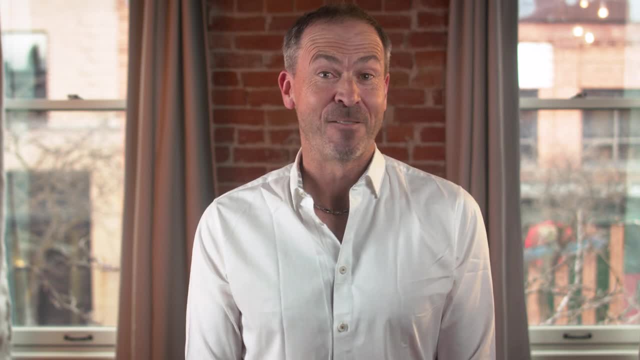 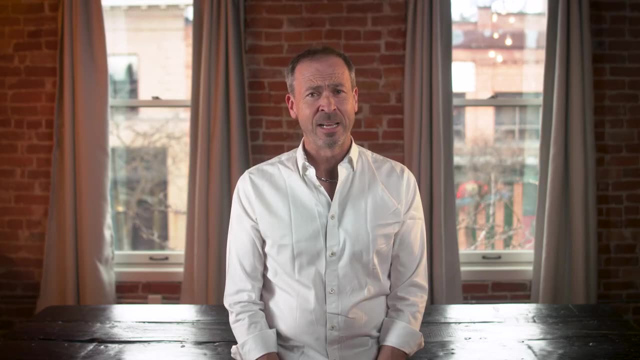 like algebra, is totally irrelevant and find it hard to focus, And if you feel like you finally get the type of problem you're working on, you might feel confident enough to read ahead to the next topic so you can keep that good feeling going. If you're nervous about a problem, you just have to bring yourself however you're. 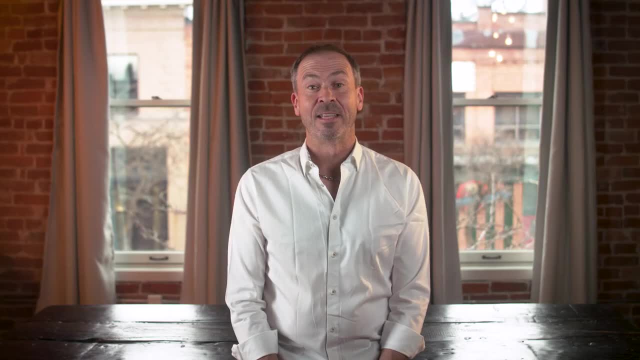 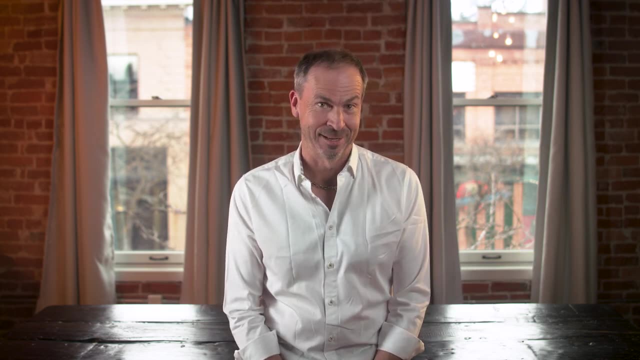 feeling. So acknowledge your reaction to the problem and then take a deep breath. And then step two is… do something, Anything. Read the question again. Read the question backwards, Maybe write down all the numbers you see in it. Just do something, whether 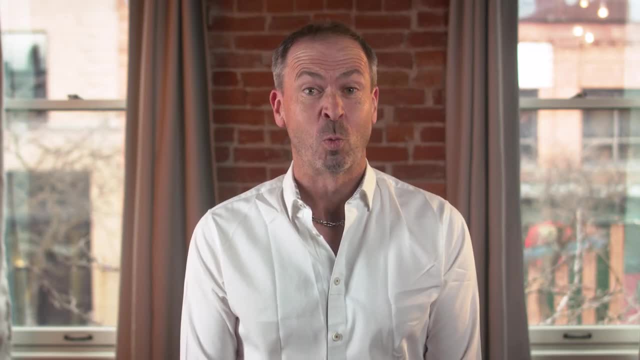 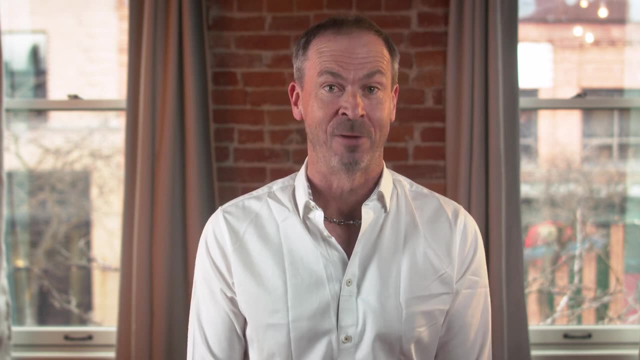 it's related to the problem or not. Now it sounds like we're procrastinating, but we'll waste a lot more time by just sitting there doing nothing, staring hopelessly at the problem. Doing something helps overcome the emotional hurdle of getting started, hopefully leading to some progress. 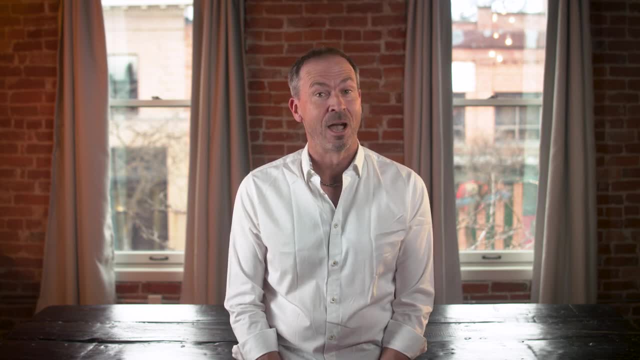 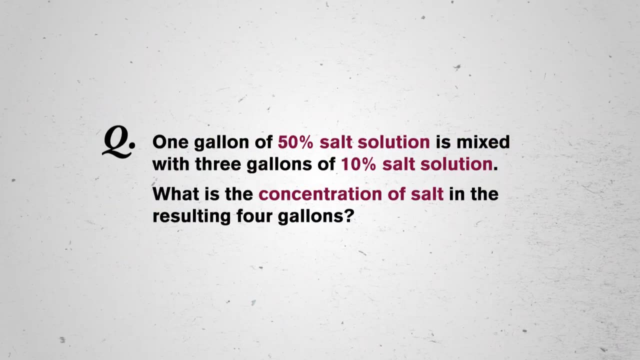 Alright, so I've acknowledged my reaction here: Nervousness. Now it's time to do something. I'm going to try drawing a picture to see if that can help me set up the problem. So let's go piece by piece and see what the problem gives us. 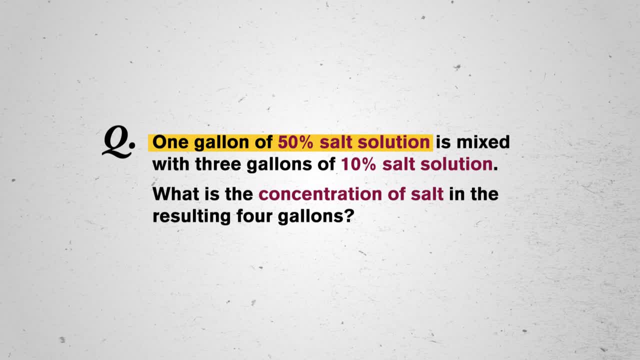 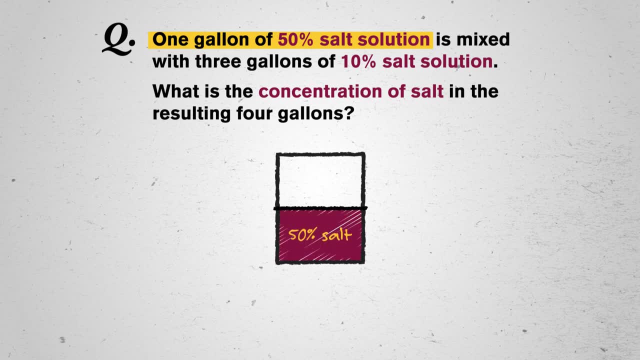 One gallon of 50% salt solution. OK, that sounds drawable. It doesn't have to be fancy. In fact, the simpler the better. So this gallon is just a block of liquid, and I know that half, 50% of it is salt. 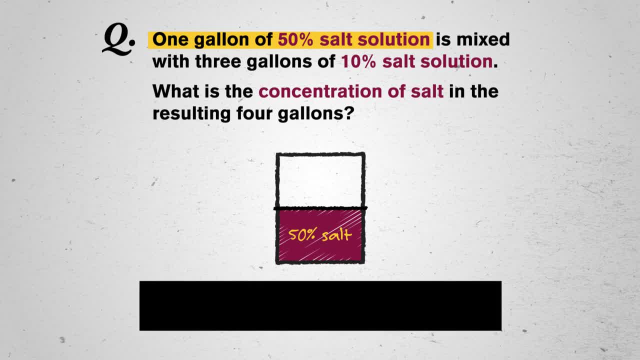 That helps me see how I could start writing a math expression. We need to think about the amount of salt. Let's call it S, So so far we have: S equals 1 times 0.5.. Half that one gallon is salt. 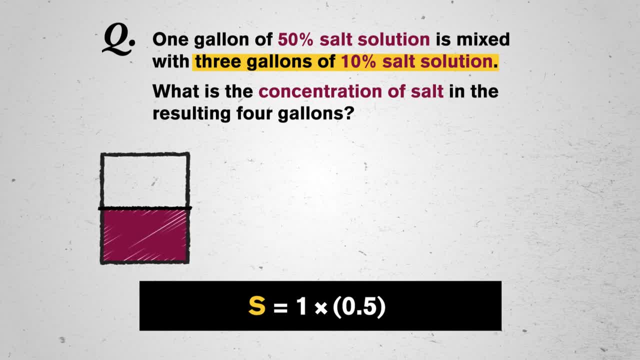 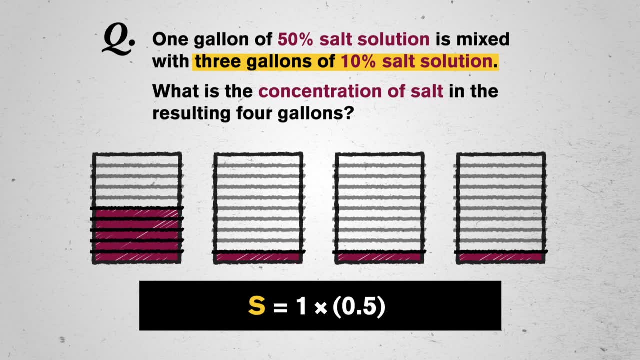 Now our first gallon is mixed with three more gallons of 10% salt. So that's three more blocks of liquid and a tenth of each is salt. Since we know we're combining liquids, we can go ahead and divide the first block into. 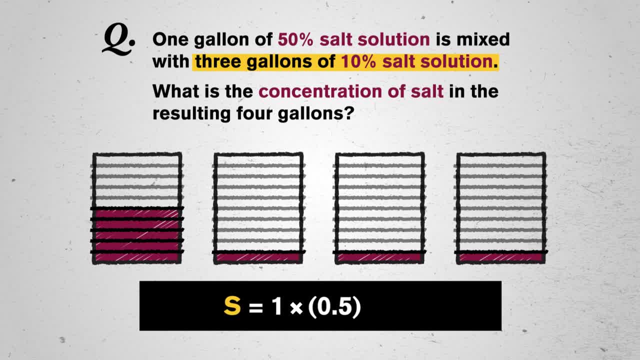 tenths to match the other gallon blocks. So that's going to add more salt to S, giving me the equation: S equals 1 times 0.5 plus 3 times 0.1.. If we work that out, S equals 0.8.. Um, hmm, is that the answer? 0.8 seems like a lot of. salt per gallon. It's almost too much. Alright, let's re-read the question and focus on what kind of answer we need to give. One gallon of 50% salt solution is mixed with three gallons of 10% salt solution. What? 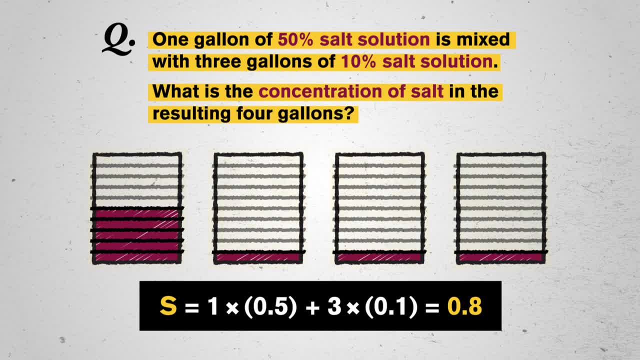 is the concentration of salt in the resulting four gallons. I already have four total gallons in this drawing, so I don't actually need to draw anything else. I just need to figure out how much of the four gallons is salt. Ah, so 0.8. 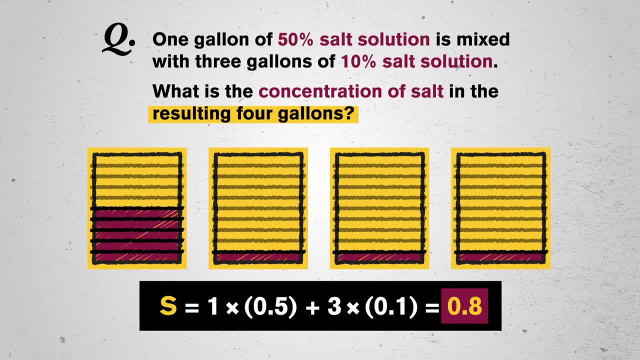 gallons is the amount of the four gallons that it's salt. Aha, now that seems more reasonable To match how the problem was written, we could translate to a percentage: 0.8 over 4 equals 0.2.. Ah, 20% salt seems like a lot of salt. 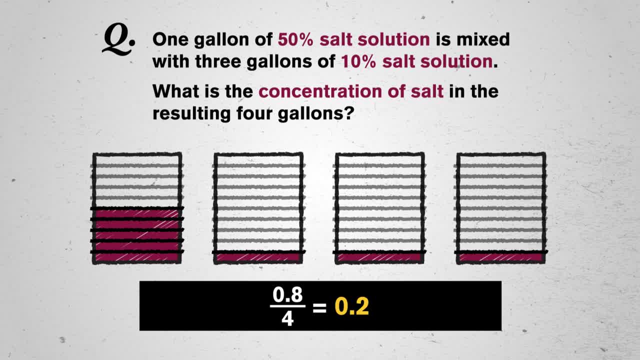 That's a logical amount for a 50% solution diluted with a lot of 10% solution, And we can check our work with our picture. I have five blocks of salt in the first gallon, one in the second, one in the third and one in the fourth. That's 8 blocks of salt out. 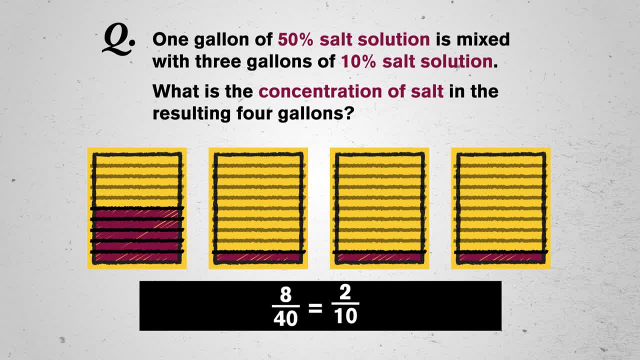 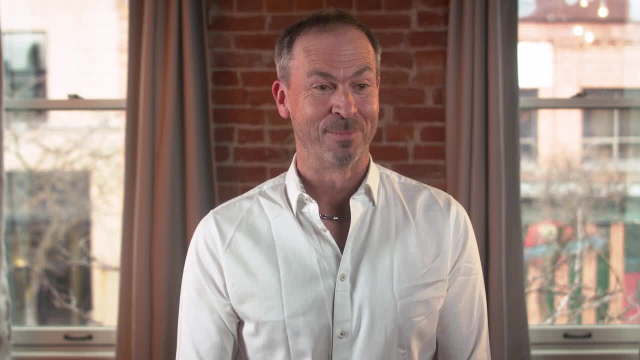 of a total of 40 blocks, And 8 out of 40 is equal to 2 out of 10, or 1 out of 5, 20%. My equations are confirming what my drawing is already telling me. Okay, let's try another one. The only way to get better at word problems is to practice. 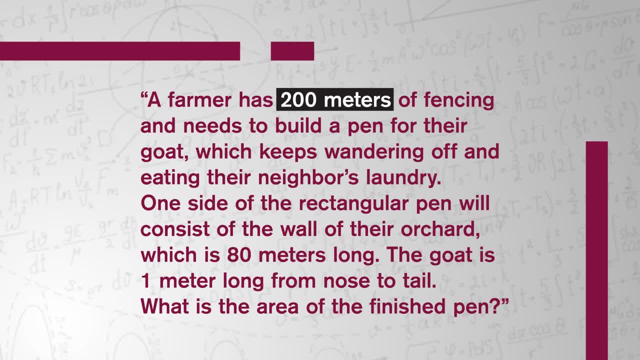 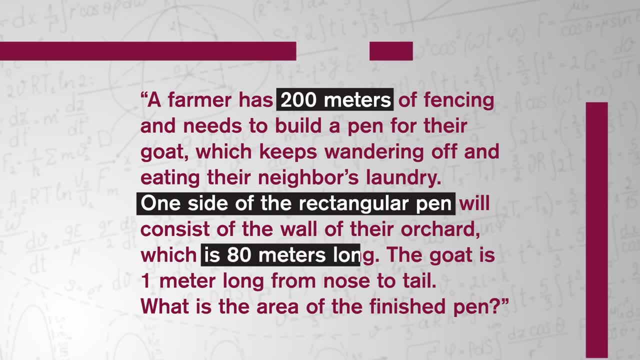 A farmer has 200 meters of fencing and needs to build a pen for their goat which gives the goat the ability to wander off and eat their neighbor's laundry. One side of the rectangular pen will consist of the wall of the orchard, which is 80 meters long. The 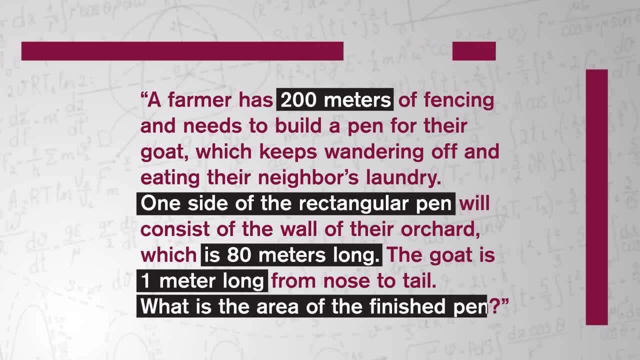 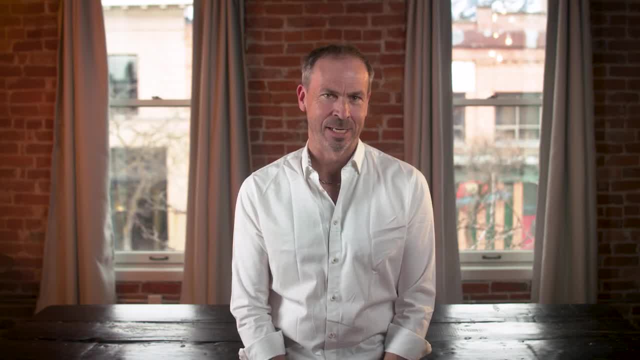 goat is 1 meter long from nose to tail. What is the area of the finished pen? Does that make for a small goat? And how much laundry could a goat possibly eat? I wish I had a pet goat, Alright. so what's my emotional reaction here? Clearly I'm daydreaming. My mind is: 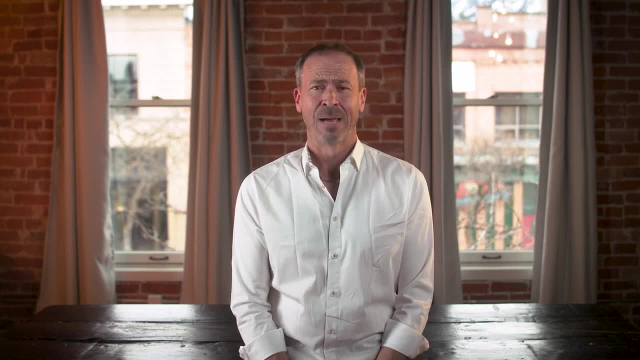 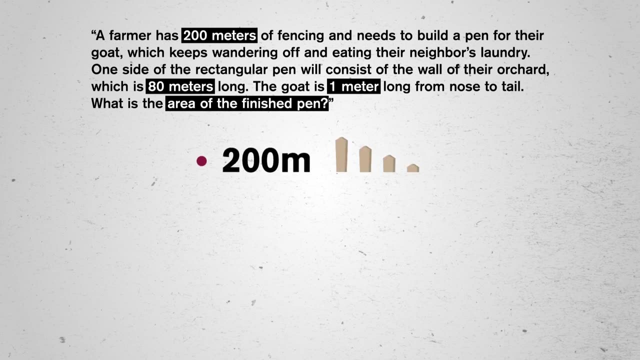 wandering. If I acknowledge that I can redirect and focus, I'm going to do something different than last time and start by making a list of the numbers we have and the numbers we want Now: 200 meters of fencing, 80 meters of wall and 1 meter of goat. Actually, do we need? 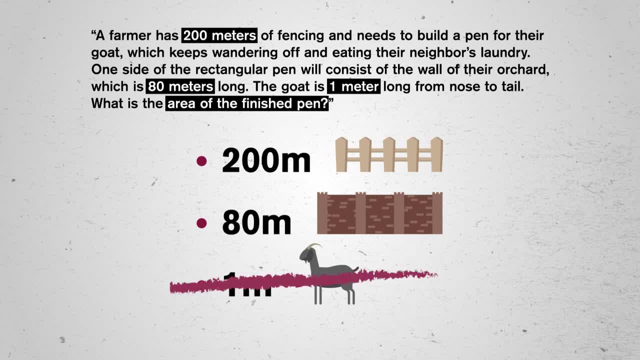 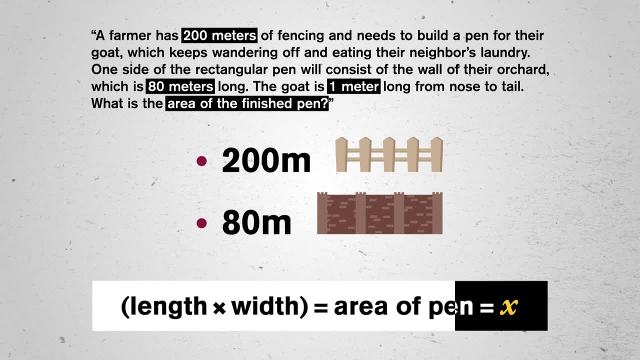 that last one. Nope, No one's ever told me to find the length of a goat before calculating the area of a rectangle, So sometimes word problems can come with extra information that won't help us solve the problem, And the numbers we want are… oh, just one number: The area of the pen. 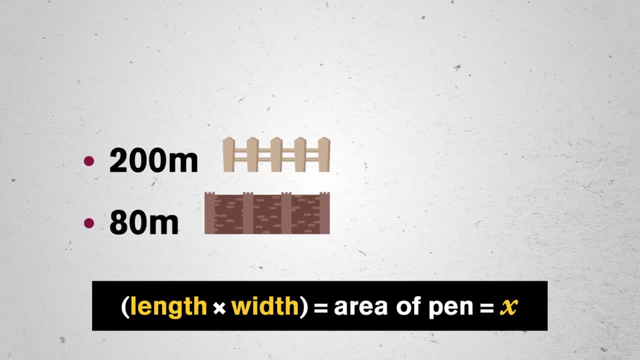 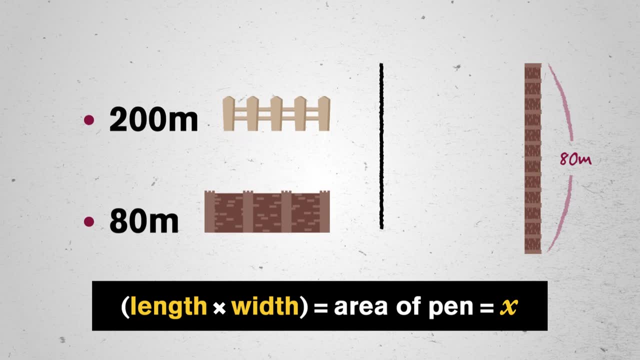 So rectangular pens, we just need length and width. Our first list shows we can call the length 80 meters, so now we just need the width. So how do we find the width? Well, we start with 200 meters of fencing and we'll use 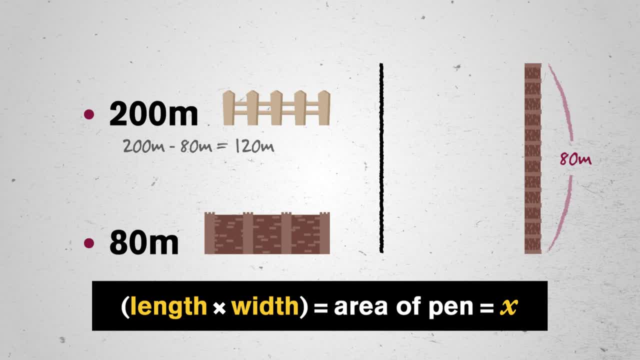 80 for the side opposite the orchard wall. So we have 200 minus 80, which leaves 120 for the other two sides, And 120 divided by 2 is 60. So let's check if that works. 60 and 60 and 80 equals 200 meters of fencing. Yes, I feel. 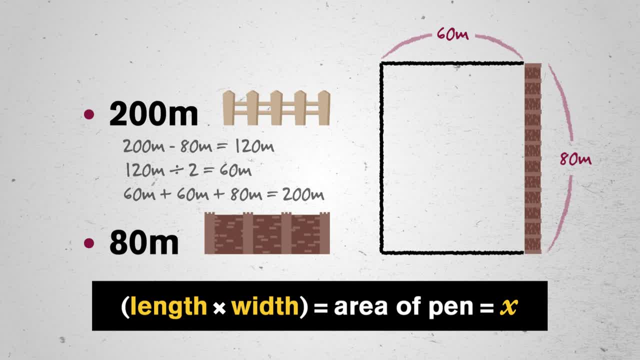 triumphant. But wait, we want the area of the finished pen, not just the side lengths. Sometimes solving a tricky bit in the problem can feel like we've solved the whole thing, But we always have to check what the question was actually asking for. 80 meters times 60 meters. 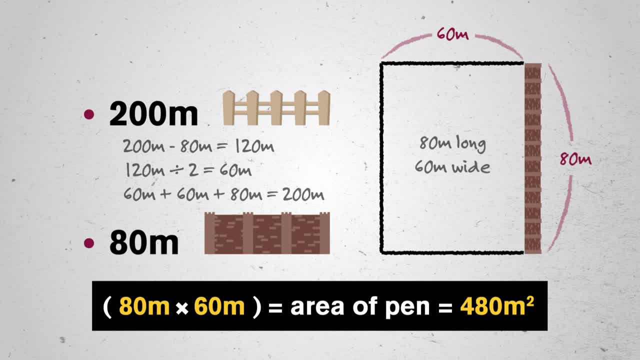 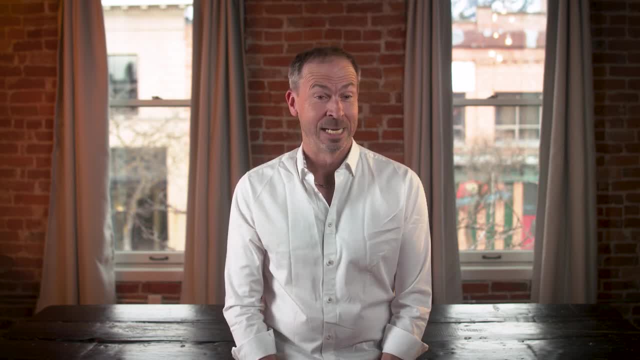 is 480 square meters. I solved this problem by gathering my information from a list of my friends and asking myself questions about what information I still needed. Now everyone claims algebra shows up in real life, but sometimes it can be quite hard to notice. Now we can put in our math goggles and use our XYZ vision to see better. So you're. 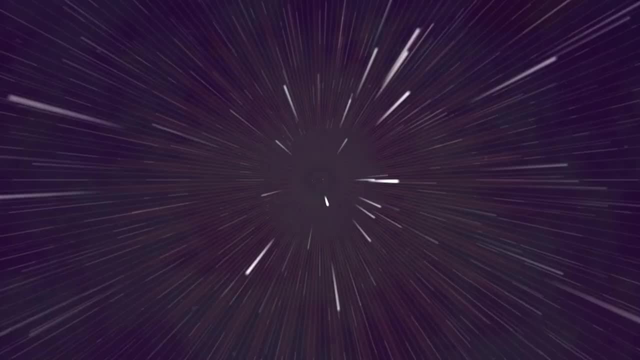 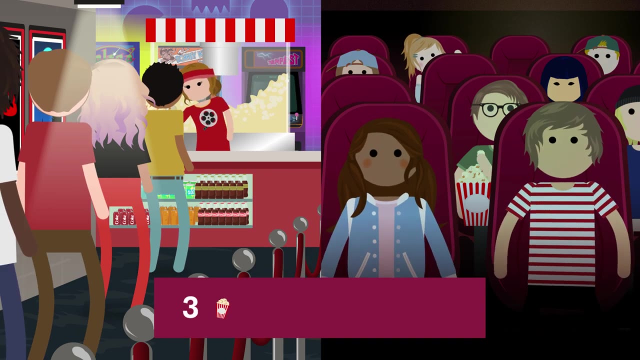 probably never going to buy 300 pineapples, but you might go to the movies with some friends. At the theatre, two of your friends picked up sodas and popcorn, while the rest of you nabbed some good seats. One friend got three popcorns and two sodas and paid $23.75. Your. 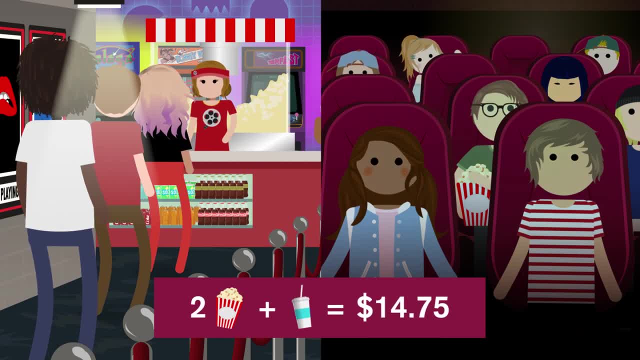 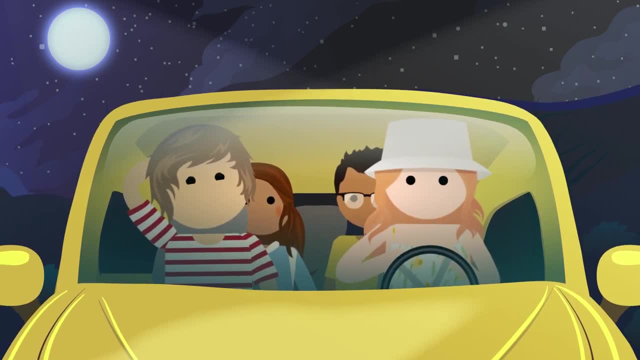 other friend got two popcorns and one soda for $14.75.. On the way home you're trying to figure out how much you owe them for your soda, But the movie theatre didn't itemize the receipts. You know you all had the same sizes of sodas. 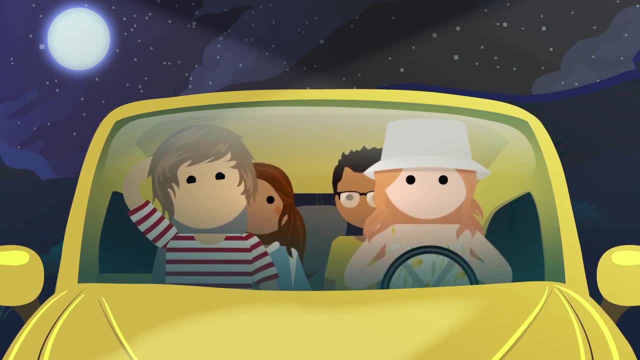 and popcorns, so it should be possible to figure out what each item costs. Equations with X's and Y's seem like overkill, but maybe you can just visualize the situation. Good thing you have your math goggles on, So you start drawing on the back of the receipt. Three popcorns and two sodas equals $23.75,. 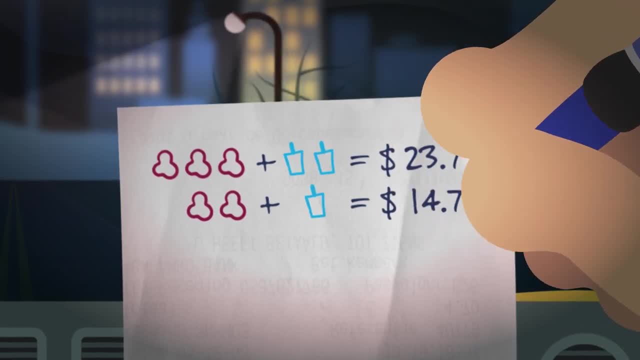 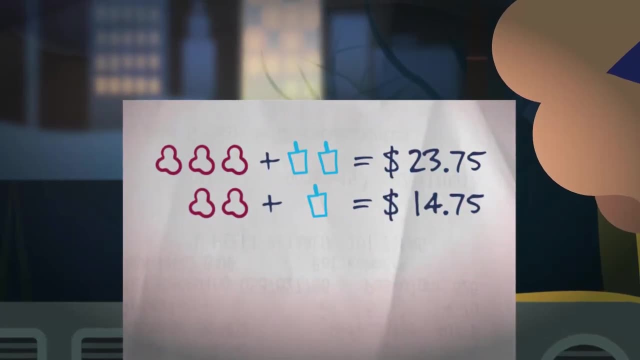 while two popcorns and one soda equals $14.75.. If you had 5,000 sodas and 3,000 popcorns, you wouldn't be able to draw a picture of the receipt, But because you have such small quantities, a quick sketch can help you notice patterns. 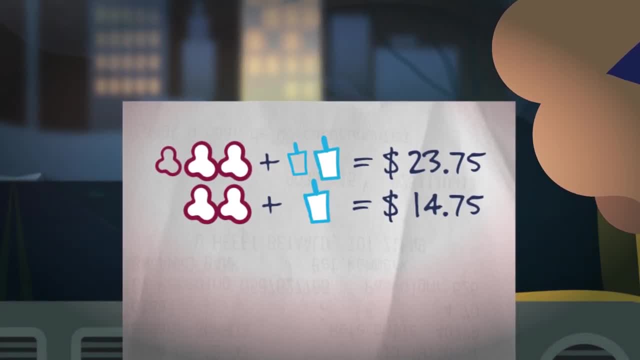 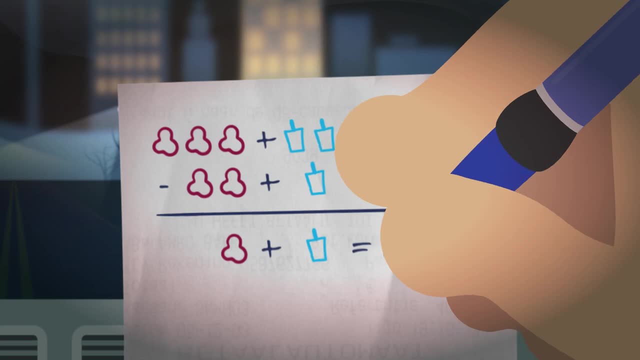 And you do In both equations. you have one soda and two popcorns And you know that equals $14.75.. Subtract the first equation from the second and you get a new equation: One popcorn and one soda equal to nine. 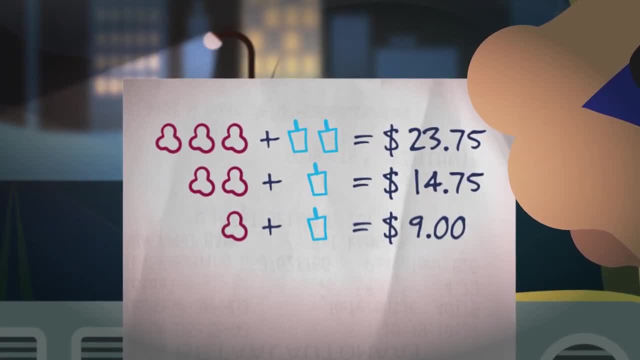 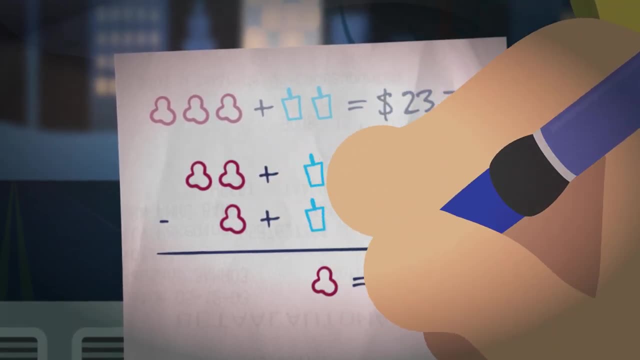 Adding that to your list of original equations helps you notice something else. One soda and one popcorn shows up in the second equation, So you can subtract your new equation from that one and see: one popcorn equals $5.75.. So close. We could plug that into any of our equations. but the third equation seems easiest.